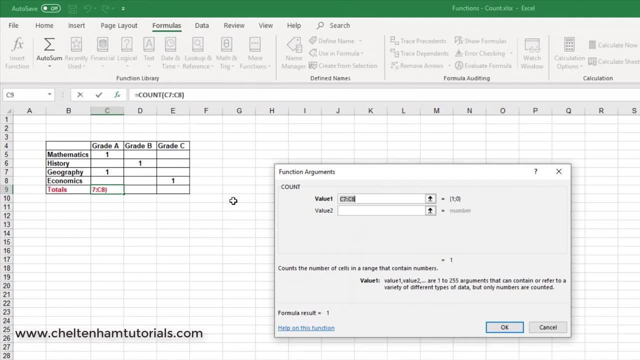 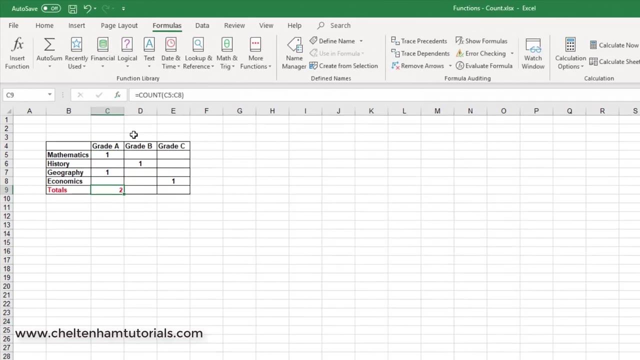 So the first thing we have to do is make sure the range is selected. So, to be absolutely sure, if we just click across there, that's selected the range C5 to C8.. Now if we just simply click on the OK button here and then click there so you can see the function, that's been inserted. 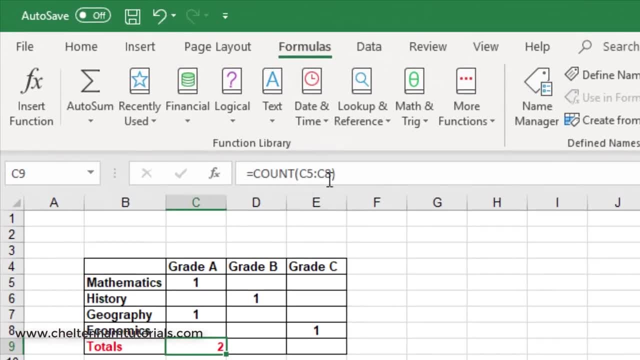 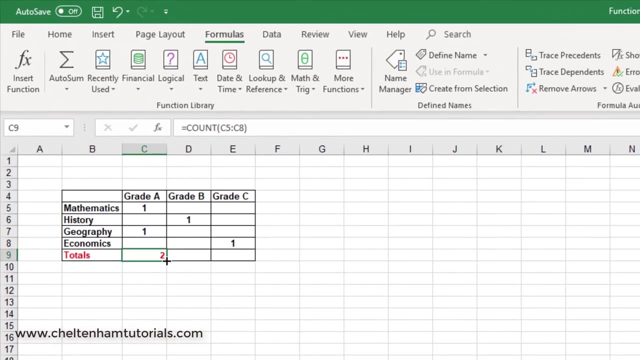 It's basically saying: use the count function across the range C5, C8, which is that range there, And it will display, or rather it will add up, all the cells containing numbers, in which case that's 2.. If I click here and go to the bottom right hand corner, then just drag that along. 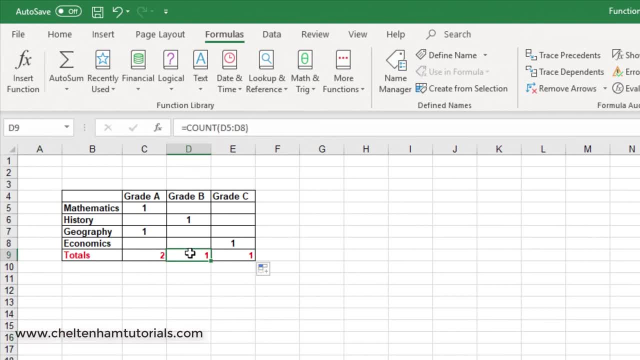 If we go here we can see we used the same thing, but for this column here, And again we used the same thing for this column here. So again in this last column it's using the count function in the range E5, E8.. 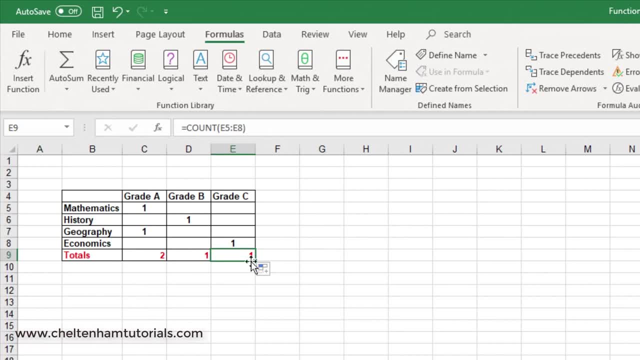 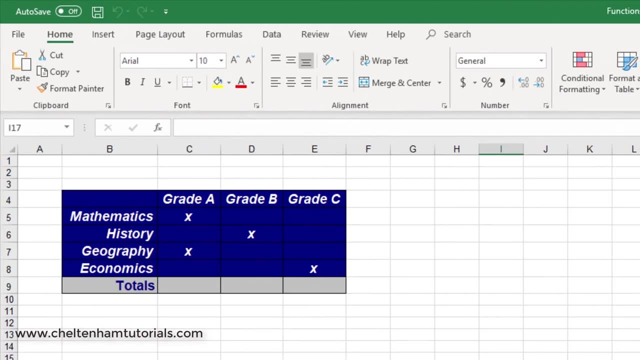 And it's basically found one number there and that displays one number. So that's how you use the count function. Now, here we're going to use the count function. So, again, similar to last time, we've got some different subjects here And we've got grade A, B, C and instead of numbers this time we've got crosses. 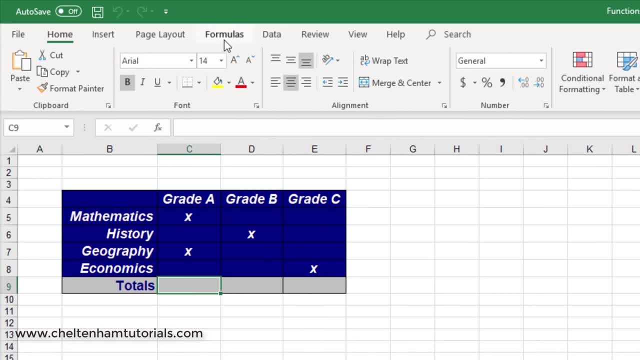 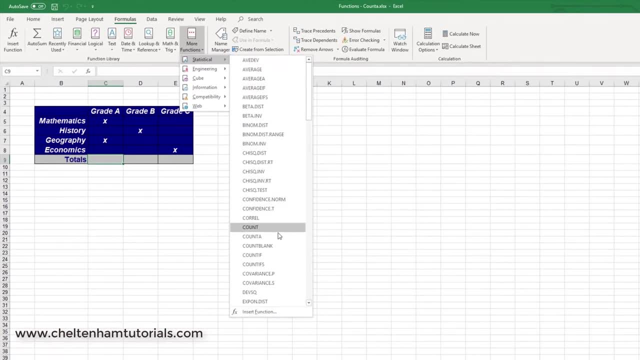 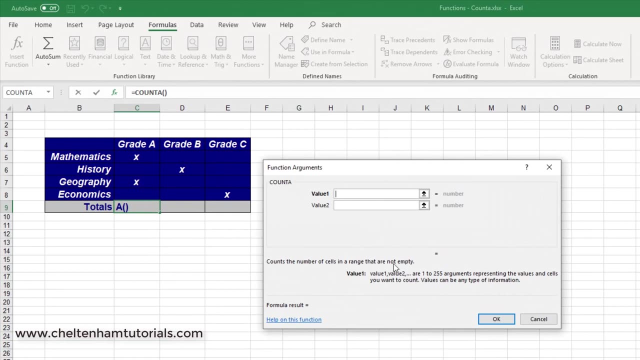 So if I click here and, like last time, I go to formulas, more functions statistical, Go down to count A, which is here. This comes up and, as you can see, this counts up the number of cells in a range that are not empty. 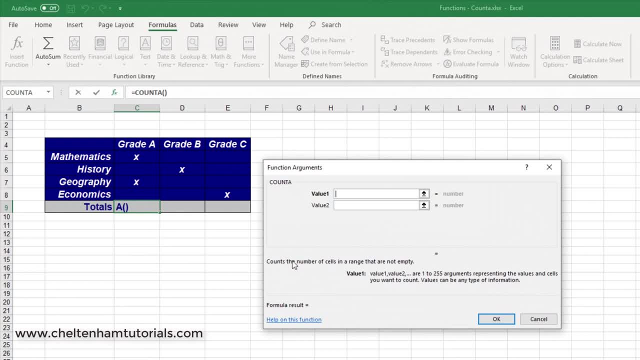 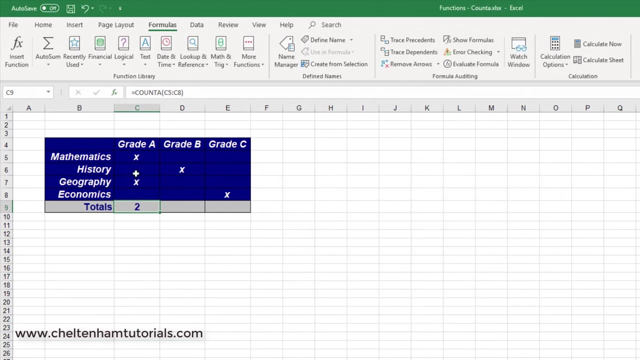 So in the last example I had to contain numbers. In this case it will just count up the cells that are not empty. So again, let's specify the range here. So I'm saying there's the range, Let's click on OK, And sure enough, that's not empty. that's not empty, so we've got 2.. 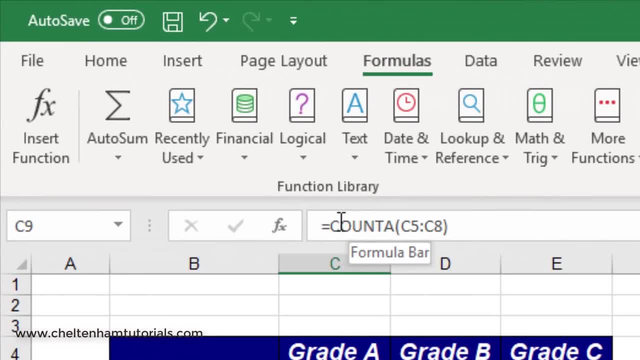 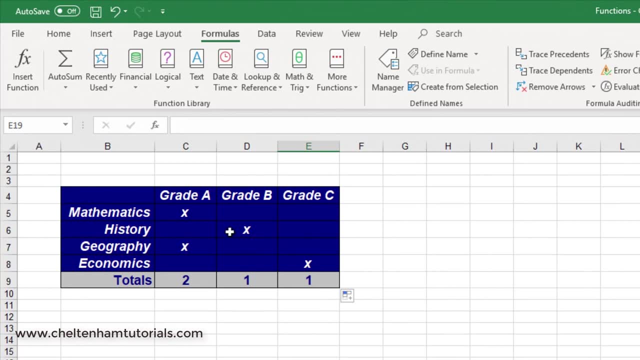 So if I click here to look at the function, it's count A across this range And of course, if I drag across here, we've got 1 in both cases, Because that's not empty and that's not empty. So that's how you use count A. 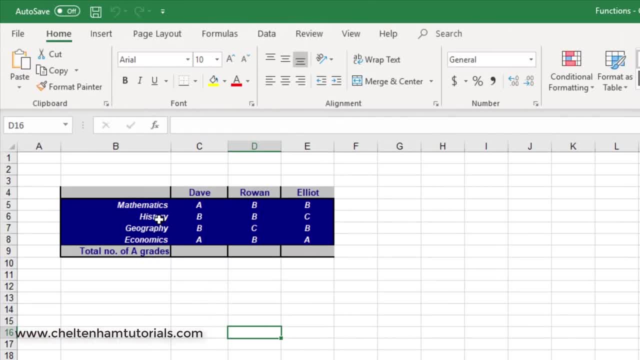 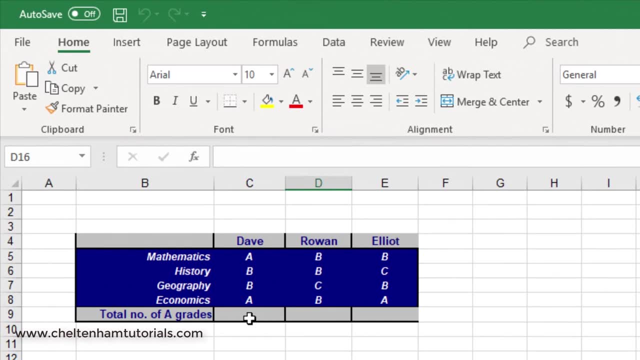 This time we're going to use the count. if So, as you can see, these are the subjects here, And we've got 3 people- Dave, Rowan and Elliot- And what I want to do here, if I click here, is I want to see how many A grades Dave has. 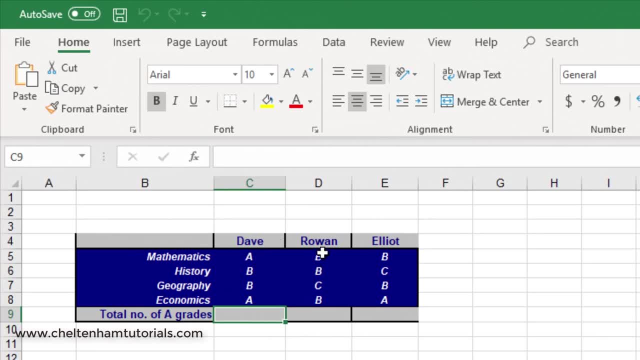 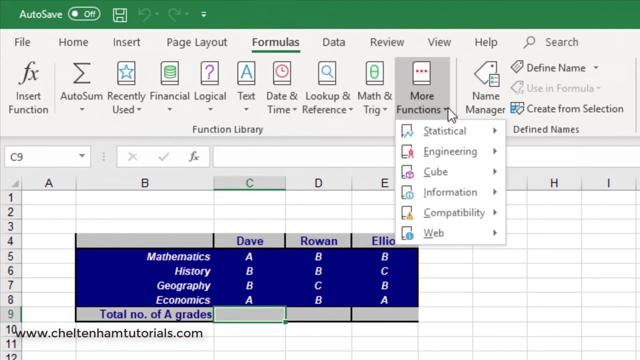 So he's got 1 and 2.. Rowan, unfortunately, doesn't have any A grades And Elliot has 1.. So what I need to do is click here. Click on Reses Formulas. Go to More Formulas. click there. 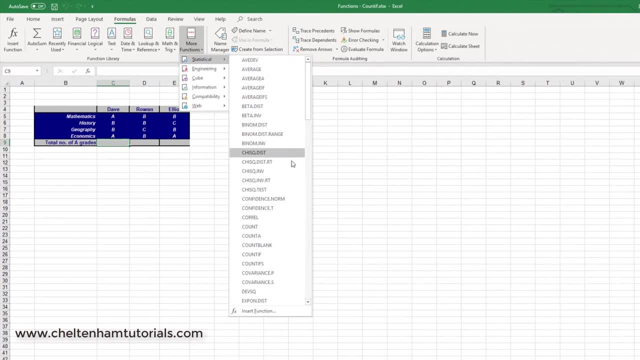 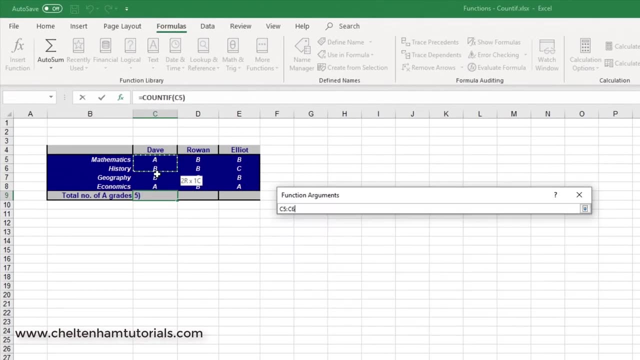 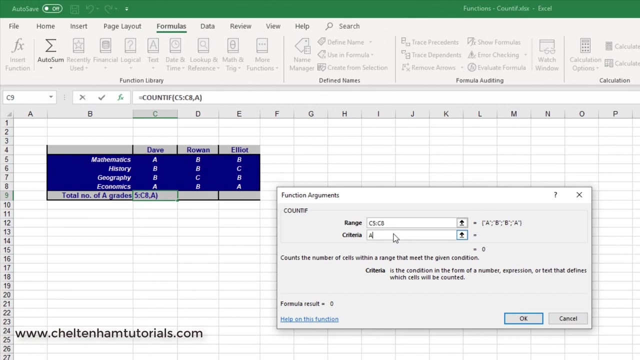 It's under Statistical. So if I scroll down I go and look for Count If, which is here. So again I need to specify the range, so I just drag across there. So that's specifying the range And the criteria is A, So let's click on OK. 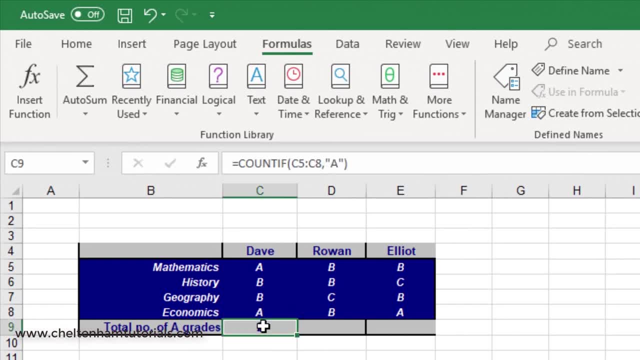 And I've got 2, which I'd expect. If we click here to look at the function, We're basically saying: use the count if function across this range And the specifier is the A as opposed to B or C or whatever, And if I drag that across here. 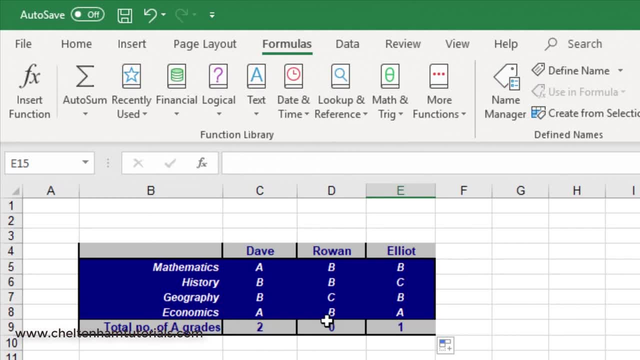 We've got 2 here because there's an A there and an A there. We've got 0 here because there's no A's, And here I've got 1A for Economics, which is displayed there. So that's how you use the Count, If function. 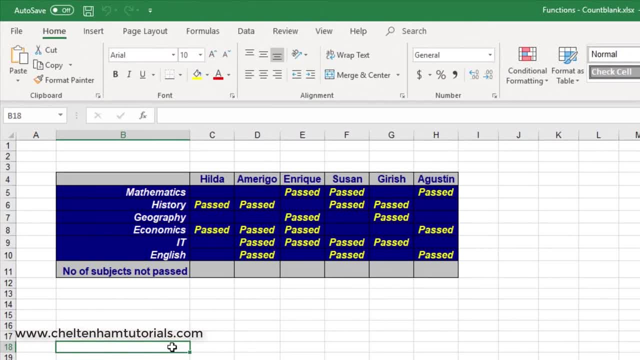 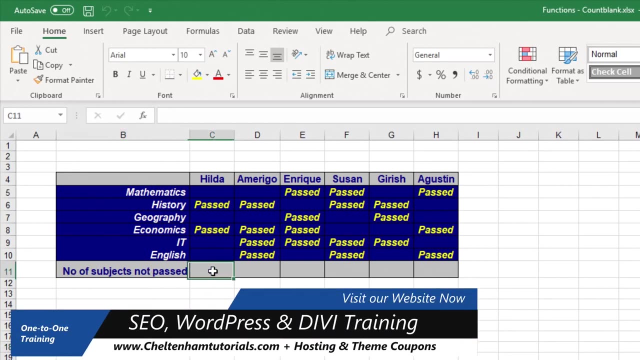 Now in this final example, we're going to use the Count Blank function. So again it's a similar sort of thing. We've got subjects down here and we've got some people across here, So this person has passed in History and Economics And I need to know the number of subjects not passed. 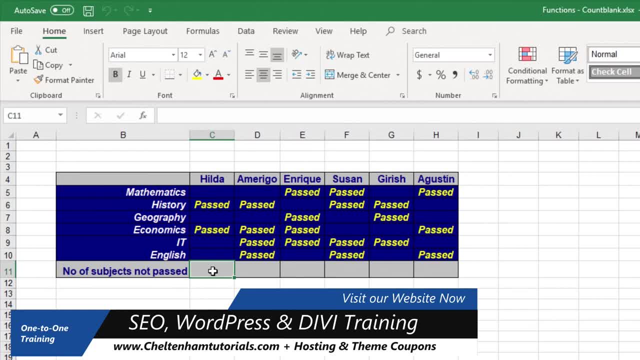 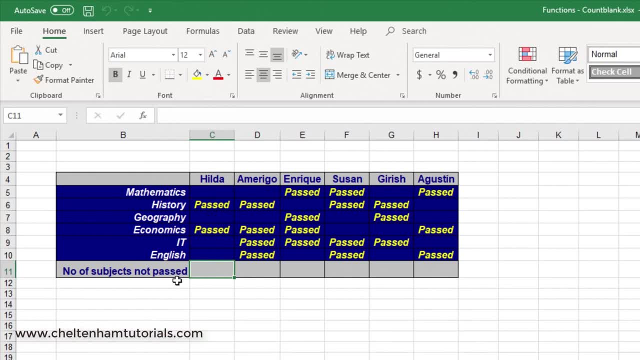 So if I click here, really what I need to do is to sum up the number of blank cells. Ie, Mathematics, Geography, IT And English. So, as before, if I click on where it says Formulas Go to More Functions. 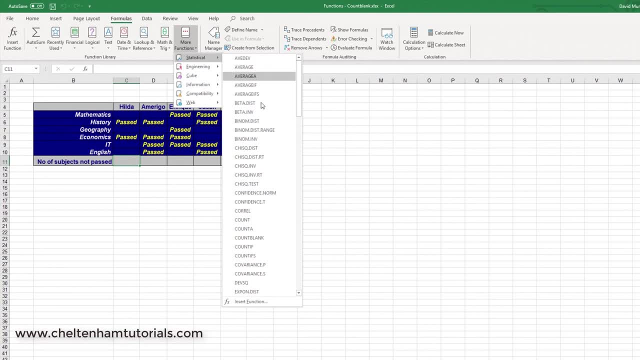 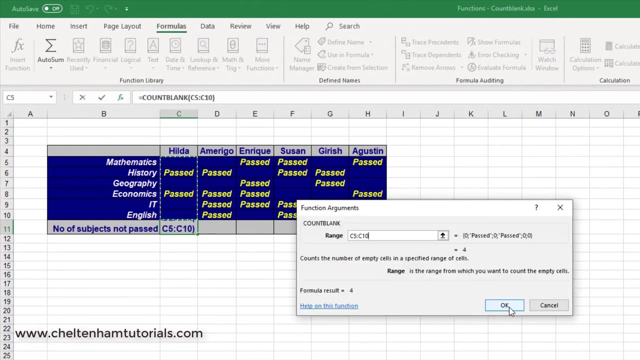 Go to Statistical And this time we're going to Count Blank, Which is there. Again, I'll specify the range And if I click on OK, You can see 1,, 2,, 3, 4.. 4 subjects were not passed.